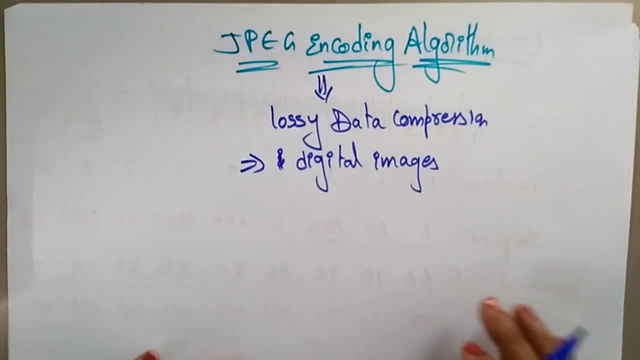 compress the file, how it is going to compress the digital image. Now let's see This. JPEG stands for? JPEG stands for: J means joint, P means photographic, photographic and E means experts, G means group. So JPEG is a joint photographic expert group. So it is a lossless 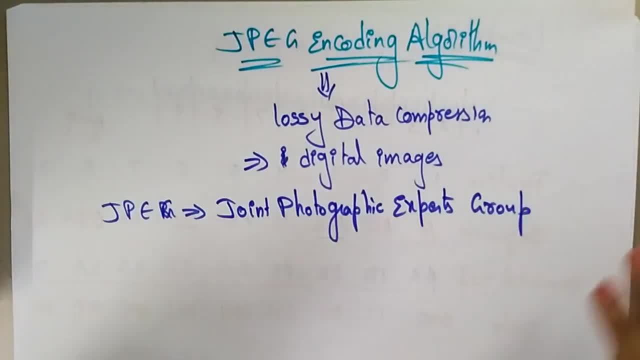 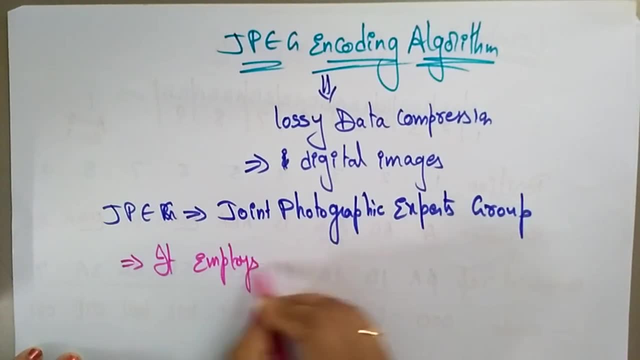 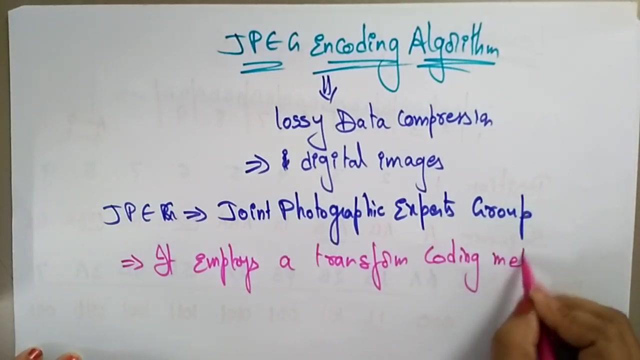 compression algorithm for digital images. Actually, what it employs? It employs a transformed code. So it employs a transformed code. So it employs a transformed code, So it employs a coding. It employs a transformed coding method. Using what technique? Using DCT technique. It? 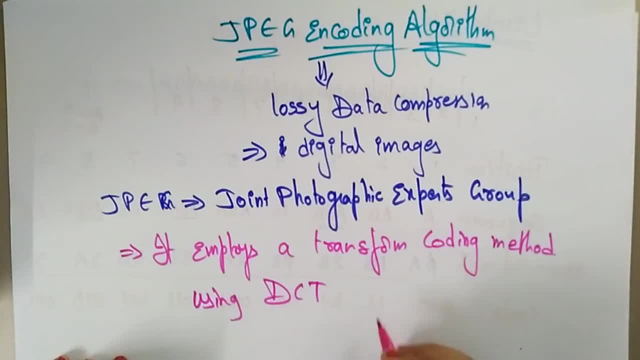 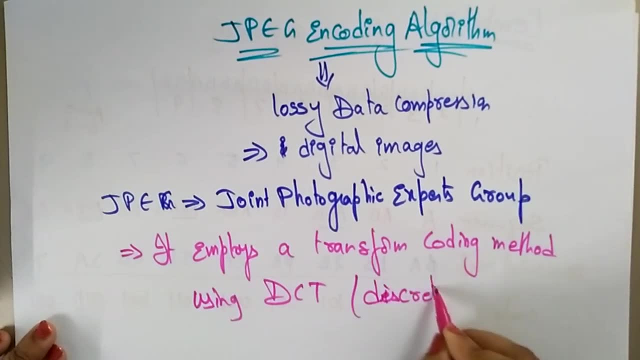 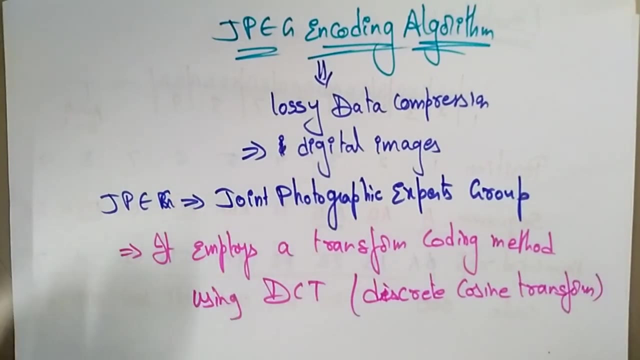 employs a transformed coding method by using the DCT technique. So what is this DCT? DCT is nothing but discrete, discrete cosine transform. So what is this DCT? It employs a transformed coding method by using the discrete cosine transform. So, by using this discrete cosine transform, it employs a 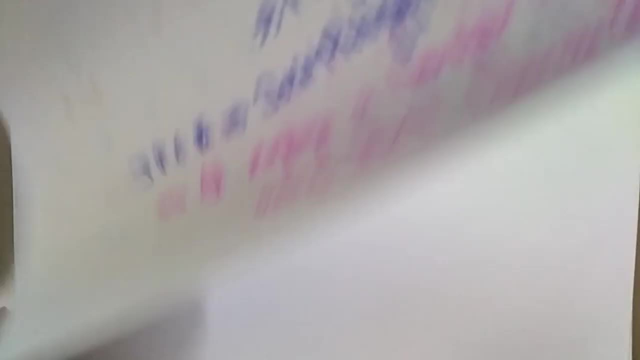 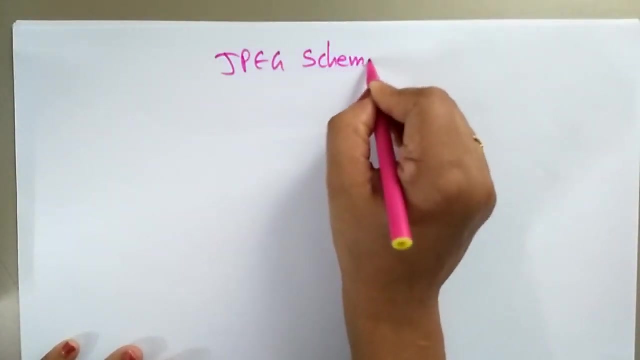 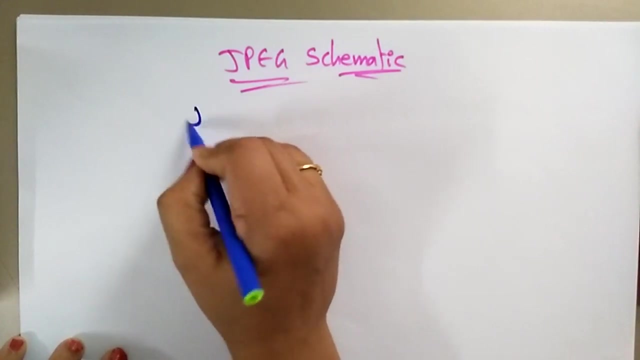 coding method. It transforms a coding method, So let me explain you how this JPEG schematic will be there. JPEG schematic. Okay, So first I want to compress the JPEG file. JPEG file: I need to compress Compression. So after I need to compress the JPEG file, So I need to compress the JPEG file. 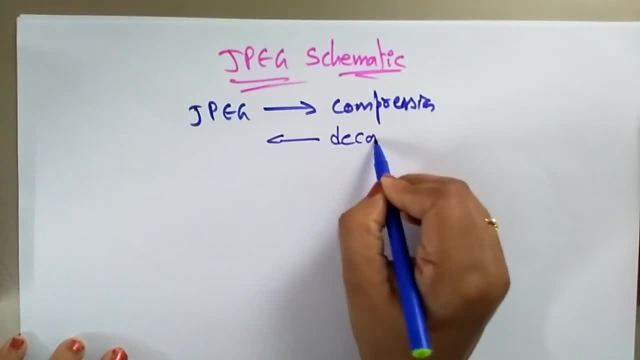 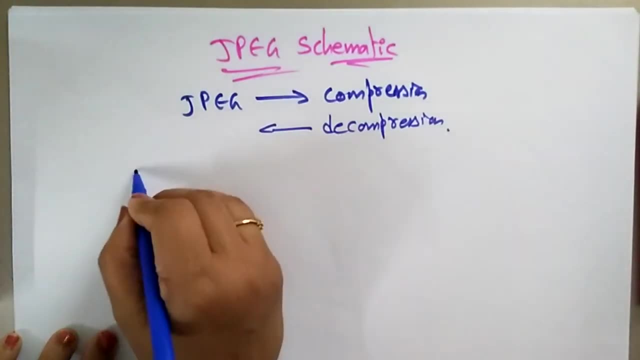 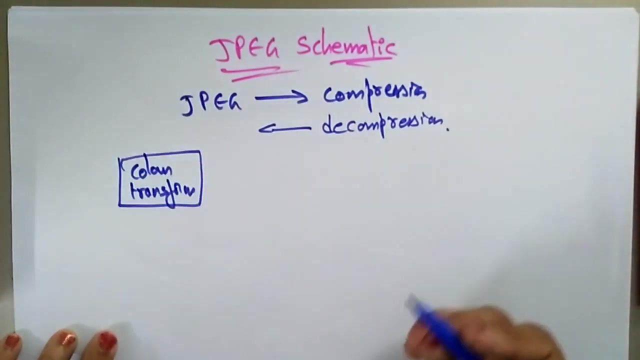 I need to decompress, Decompress, So this is my aim. So, first, what I have, what it is doing: It takes the color, transform. So we are talking about the images. So images means obviously they are in color. It's a red, blue, green color, But JPEG will take another format of color. Okay, Instead. 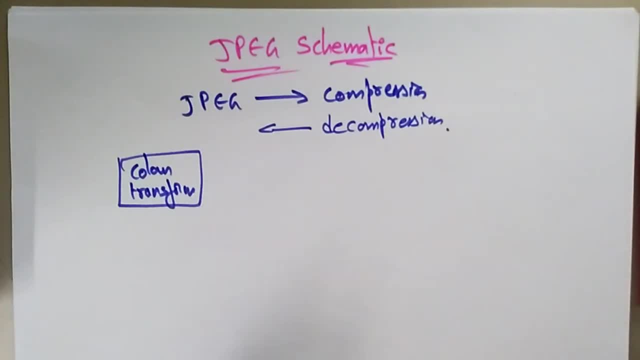 of red, blue, green, it will take, it will convert it into Y, C, D, C, R. Okay, So I'll explain later, But first it takes the color transform. So it is going to transform the RBG. 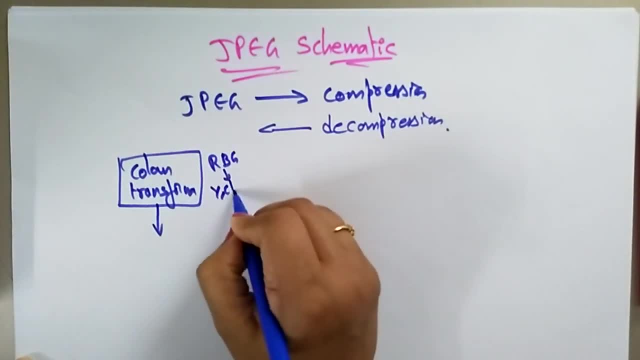 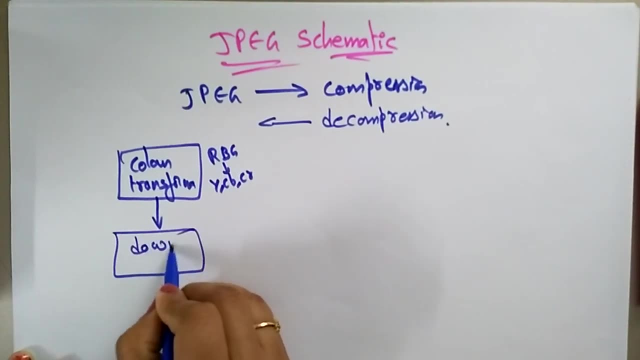 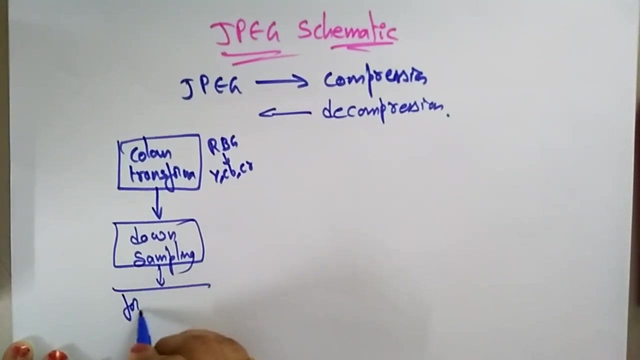 red, blue, green, color to Y, C, B, C, R. Okay, So color transform. After that it is doing down sampling, Down sampling. So then apply the DCT technique. That is a forward DCT technique. 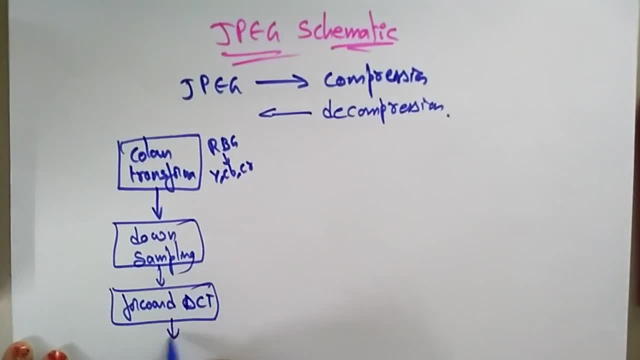 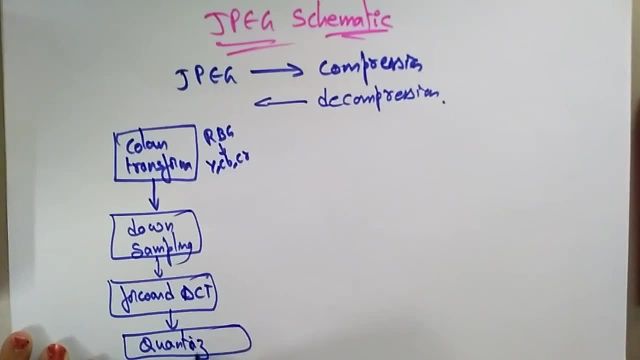 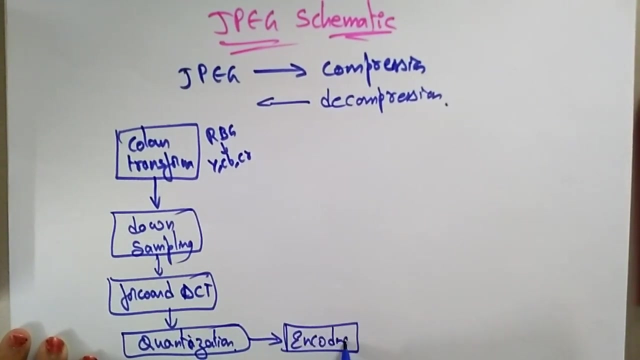 This discrete cosine transform, Then it quantizes. Quantization process will be there, Quantization. Then after that it starts encoding, Then after encoding, compress the image data. So whatever the image that is there, it is going to be compressed Image data. So up to here the compression will be over. 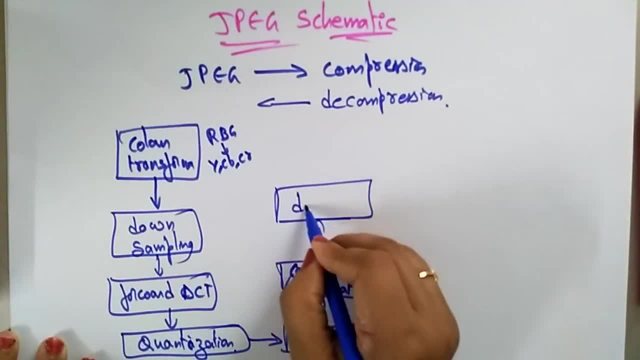 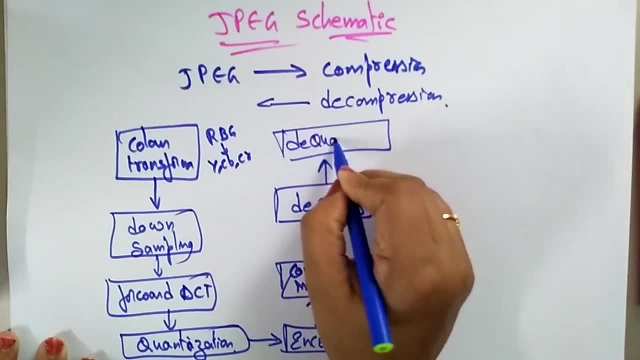 After here, the compression will be over. After here, the compression will be over. After that, again, I want to decode it, Use the decoding technique. So for decoding, you need to de-quantization. So whatever the quantization is applied that you need to be. 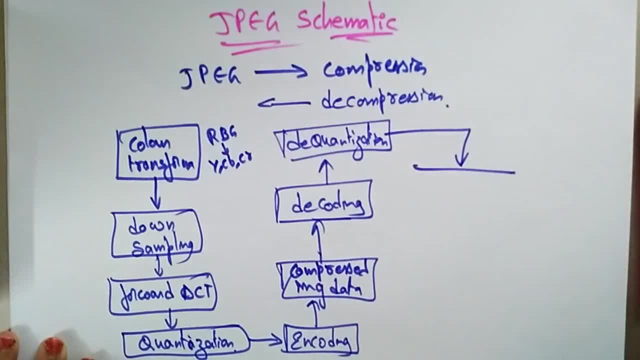 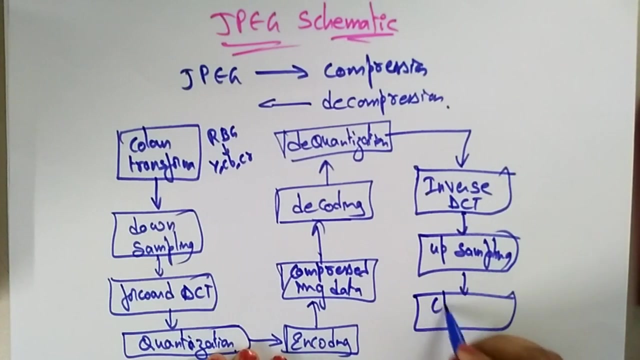 de-quantization. So now you have to forward DCT, apply the inverse DCT. So this is for decomposition. Decompression, Then up sampling. You have to do the up sampling, So this is for sampling And finally you will. color transformation has to be again performed, Color transform. 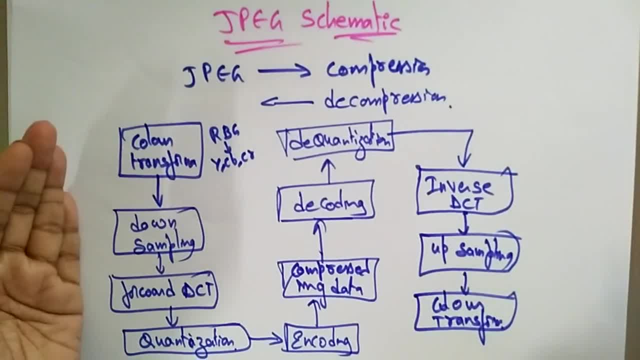 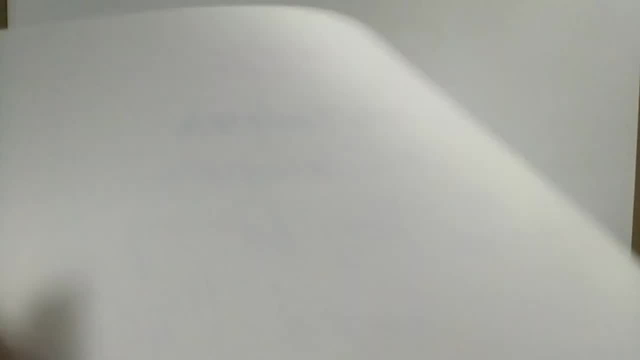 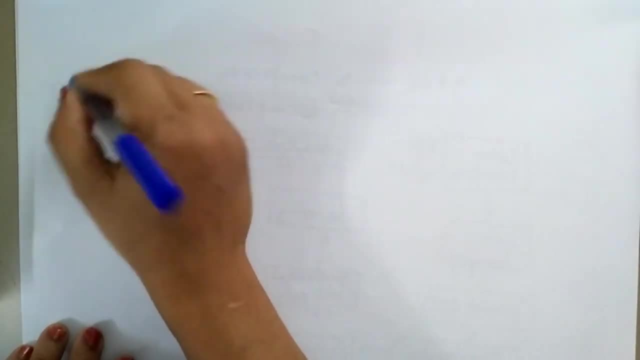 So this is all about JPEG decompression, And this is compression and this is decompression. So this is completely as JPEG schematic, Okay. So let me explain you the algorithm. So afterwards I will explain an example of how the JPEG is encoding. 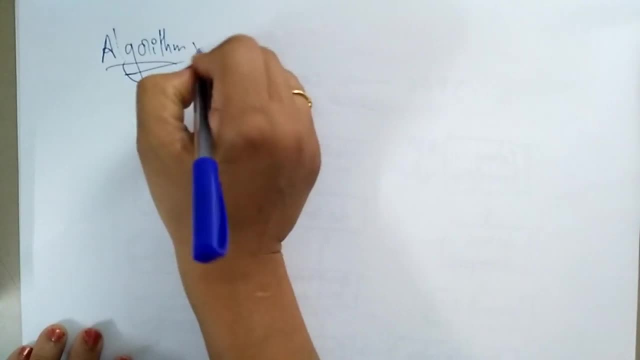 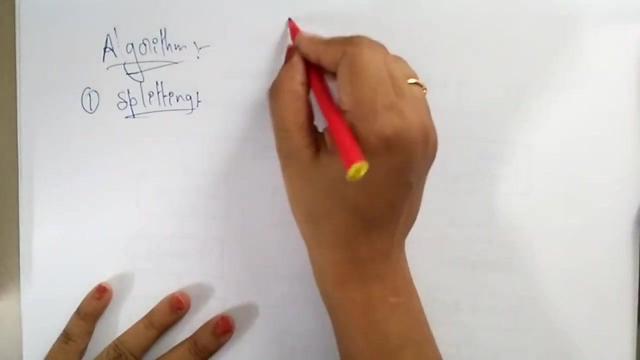 algorithm. okay, so first, what it is doing, i have to color transform. i have today before. that first is splitting. so whatever the image that is there that you need to be split, you have to split that image. so original image is there that this is. let's take: this is an original image, a i need. 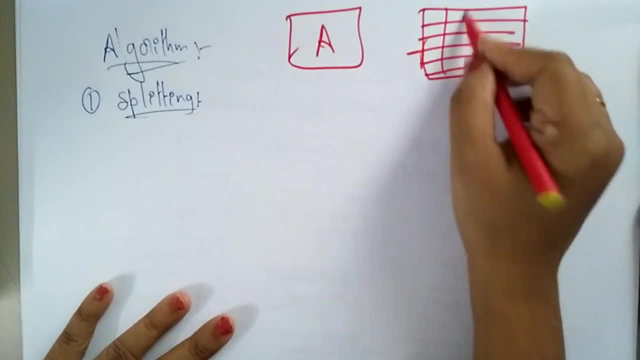 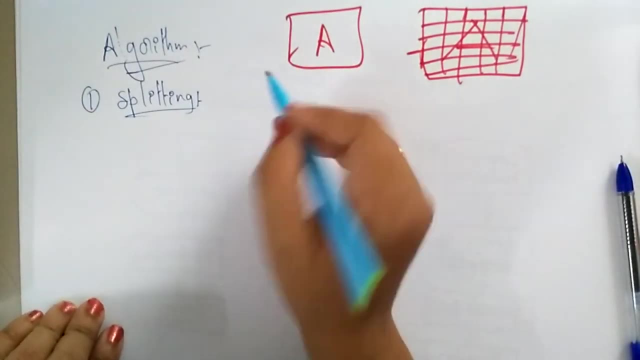 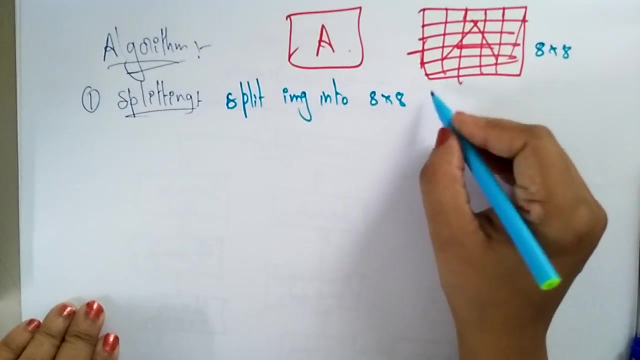 to split this original image. okay, so for that what i am doing, let me let me explain: split. split the image into 8 by 8. this is an image. i am splitting this image into 8 by 8. split image into 8 by 8. matrix: non-overlapping pixel blocks: non-overlapping. 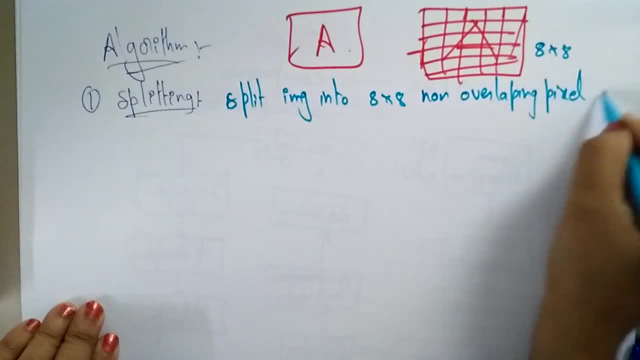 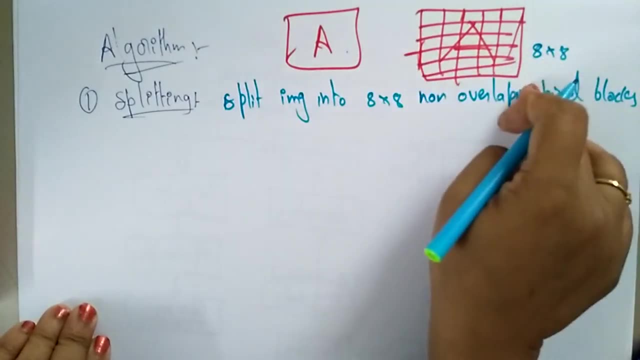 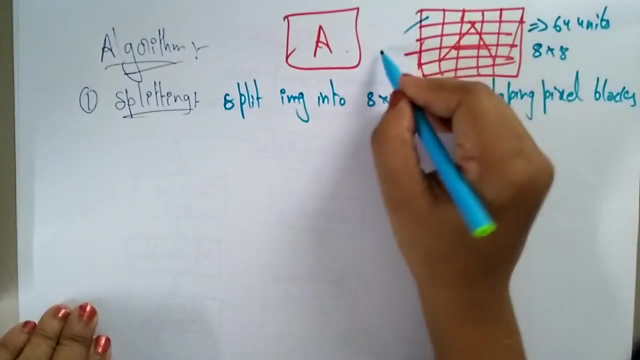 pixel blocks. so whatever the image that is there that i splits into non-overlapping pixel blocks, that is, the 8 by 8 means total 64 units are there. so here, 64 units are there. each unit you call it as a pixel. just remember that, each unit, you call it as a pixel. so if the image cannot be divided into, 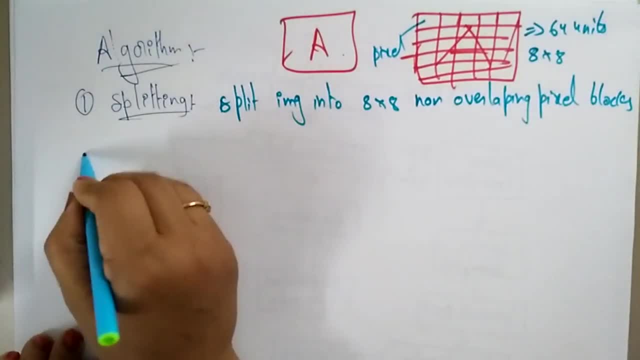 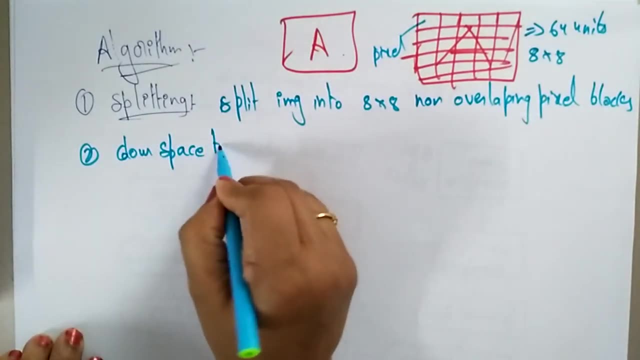 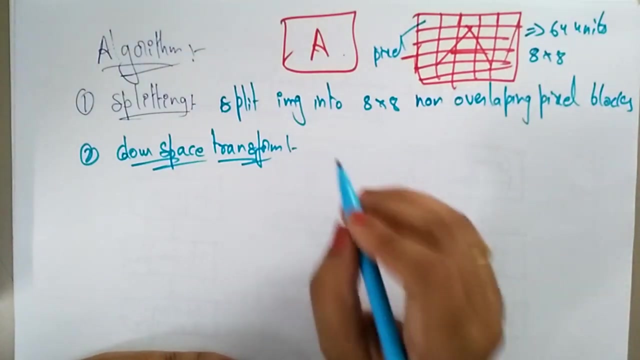 8 by 8. you can add some more blocks here. and next, color space transform. color space transform. color space transform. so why i am doing this color space transform? because if you want to convert the compress the file, the jpg will take here. color space transform from rgb, red, green, blue color to y, cb, cr. so here: 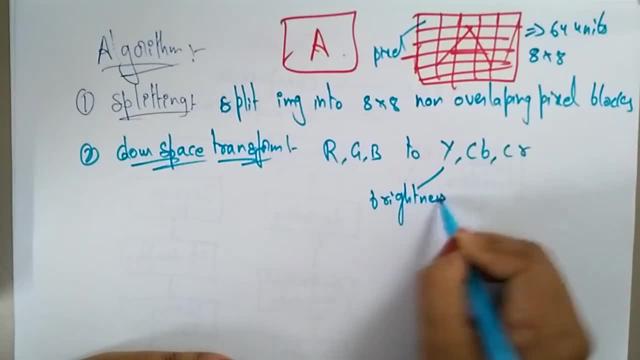 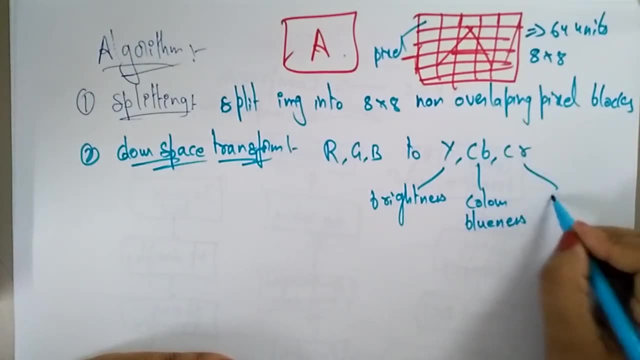 y is nothing but the brightness, cb is nothing but the color blueness. color blueness and cr is nothing but color redness. so instead of rgb, it is first. it transforms the color into y, cb, cr. okay, so actually rgb is a simple color space model. 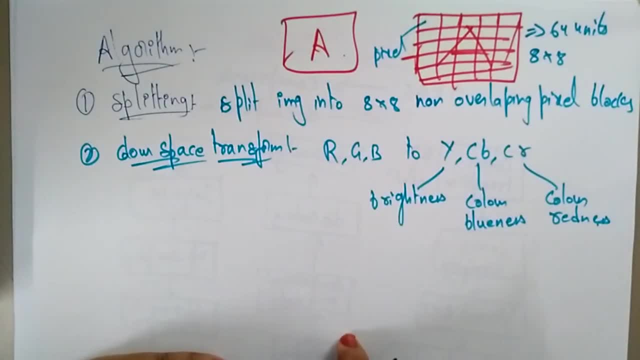 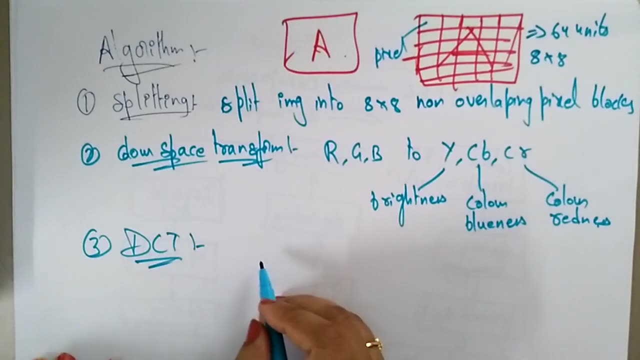 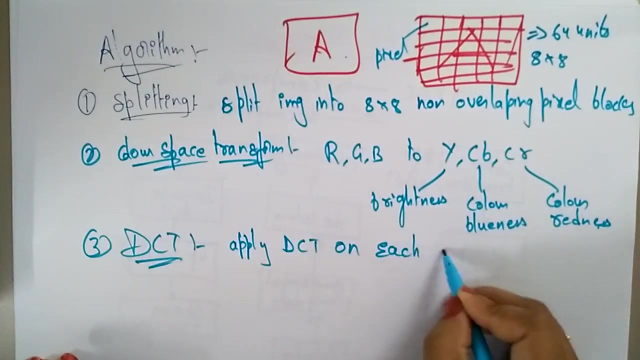 and that will be converted into this: uh, y, cb, cr. okay, after that, what i had to do? the next step is apply the dct. dct: a discrete cosine: transform it. takes the dioxide: take discrete cosine: transform for of each eight by eight block. apply dct on each. that. take discrete cosine: transform for of each eight by eight block. apply dct on each. 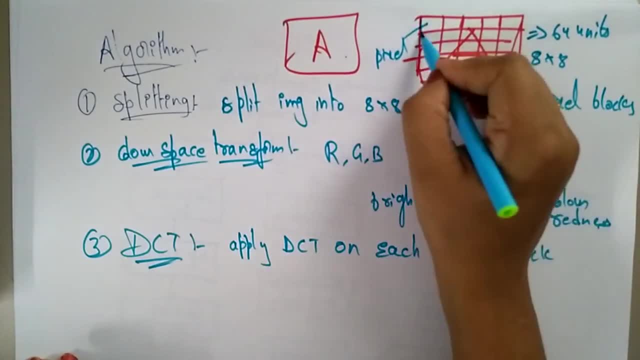 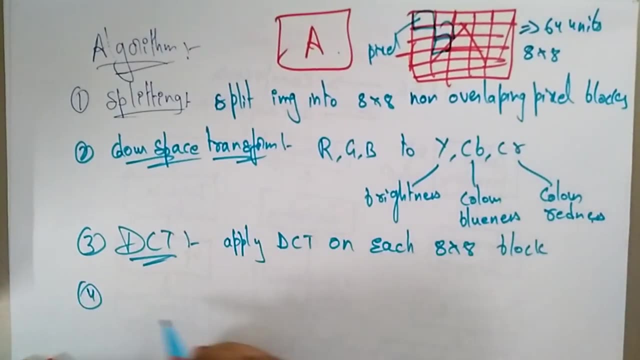 8 x 8 block. so apply on each 8 by 8 block. so apply on each 8 by 8 block. next, 8 x 8 block. next, after that, according to the schematics, what i have to next is quantization. after that, according to theよね: 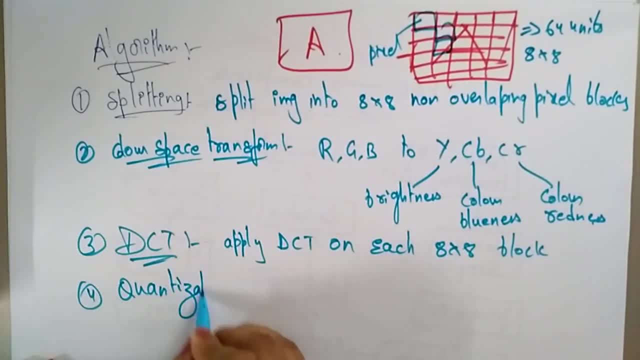 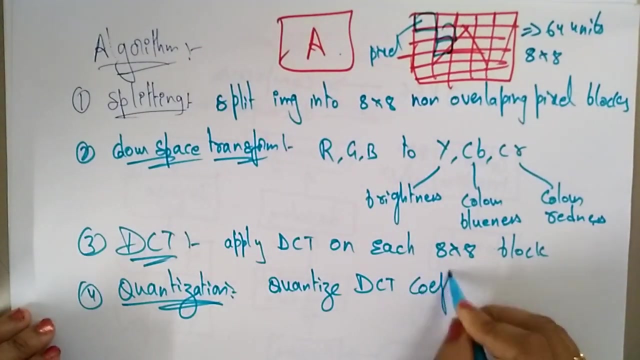 quantitation. apply quantization quantization. it quantize the dct coefficients according to the uh, psycho, visual, time quantization table. so you have to quantize the dct, quantize dct coefficients according to the okay, so according to the psychological, psycho, visualize, visually tuned quantization tables. 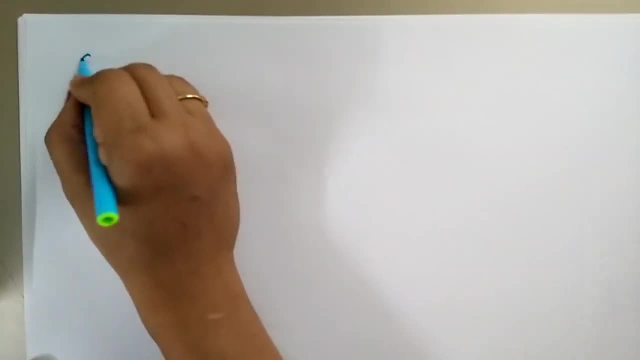 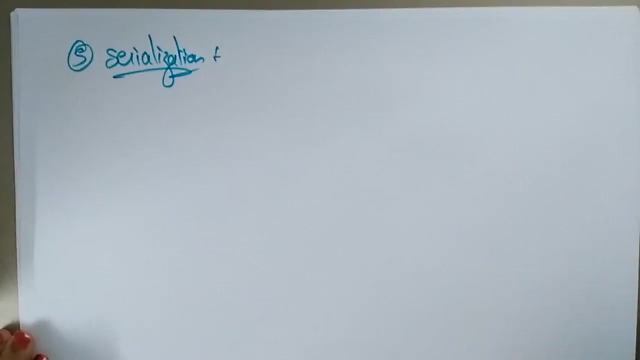 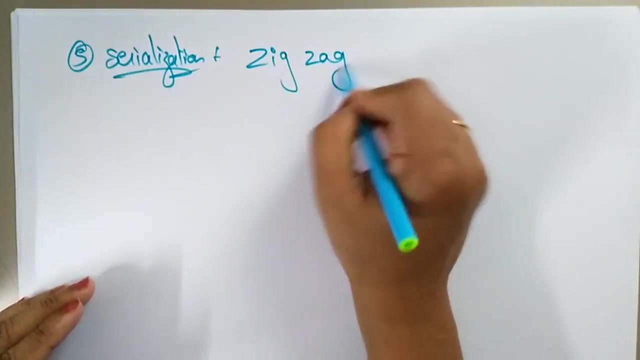 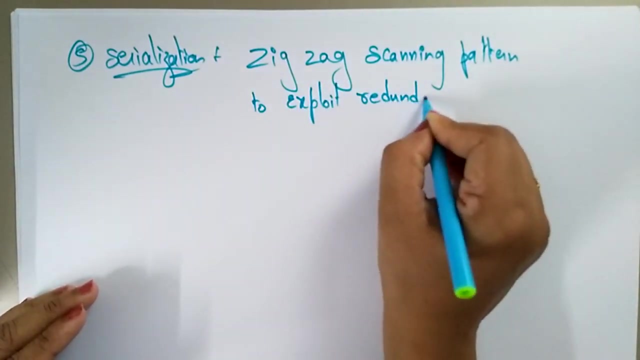 so after quantizations, you need to serialize serialization. okay, here serialization, we are applying the zigzag scanning pattern. zigzag scanning pattern. why we are applying zigzag scanning pattern? to exploit redundancy, to exploit redundancy. so for that case, we are using the zigzag scanning pattern for the quantization. 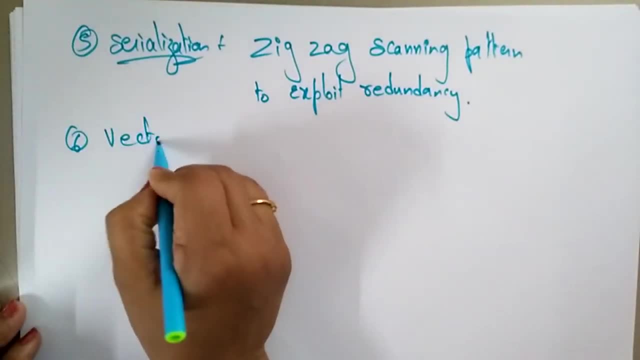 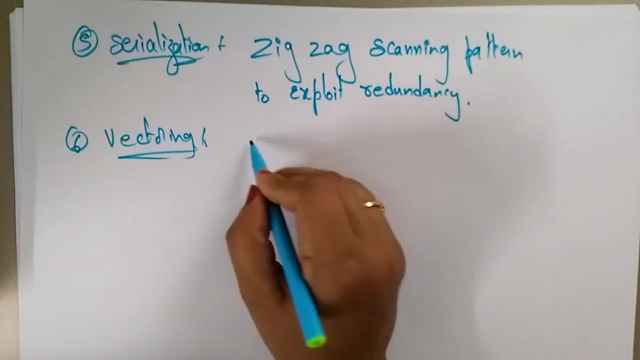 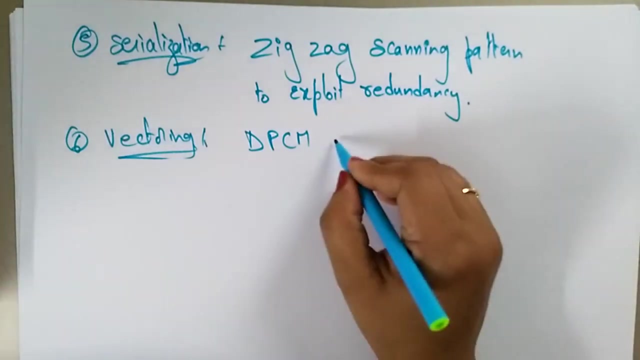 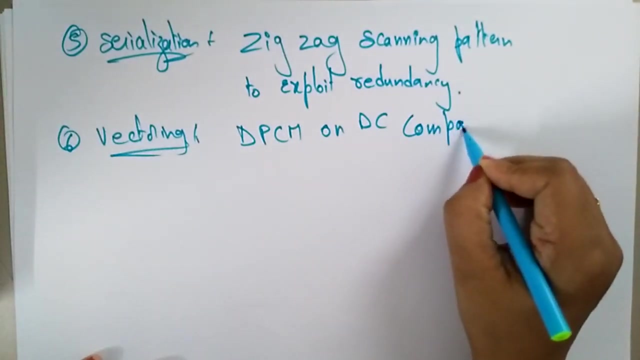 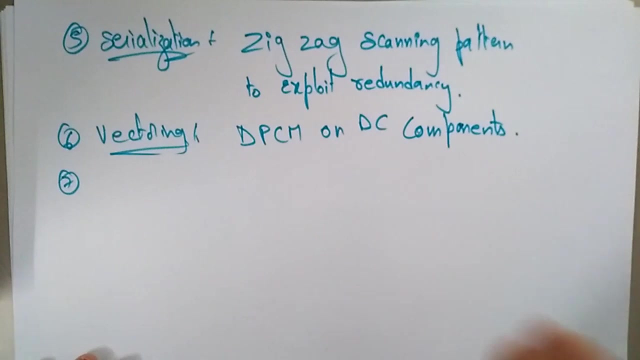 okay, so next vectoring. after that you need to perform the zigzag. scanning is over, you need to vector. it means differential pulse code modulation, that is, apply the dpcm- differential pulse code modulation on dc, on dc components, on dc components. so next run. so after doing everything like this means series is zigzag. 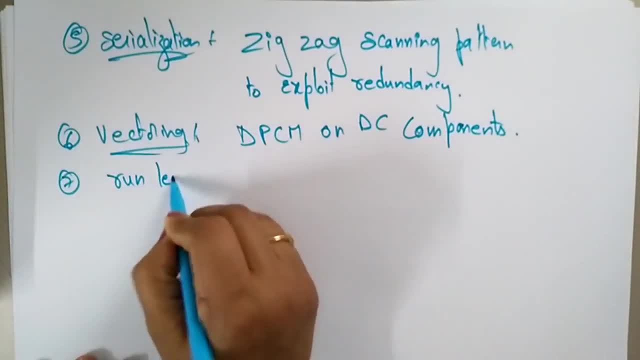 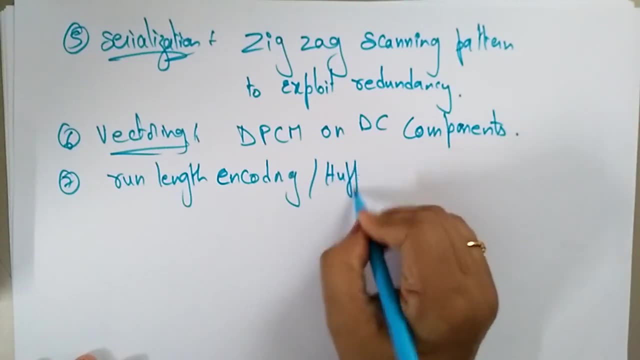 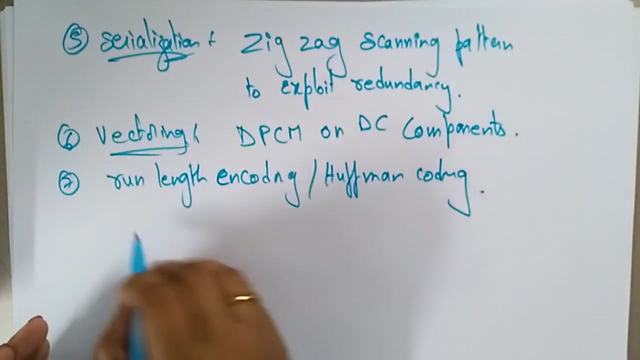 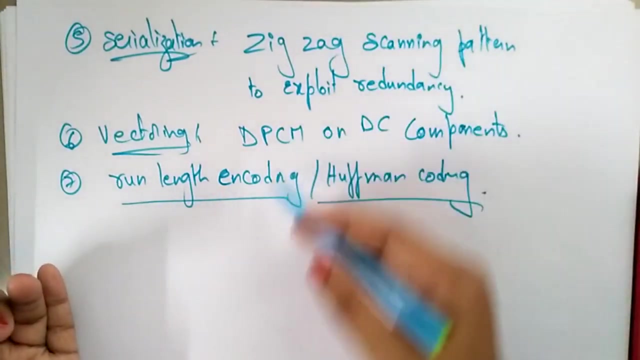 pattern, apply the run length algorithm. okay, you can apply the run length, or coding, encoding, or halfman coding, whatever it may be. you can apply that technique, the same procedure. so here you already know how to apply run, run length and encoding, so to make the data, uh, in this formatted. you need to do all these things because this is an image, not the character. 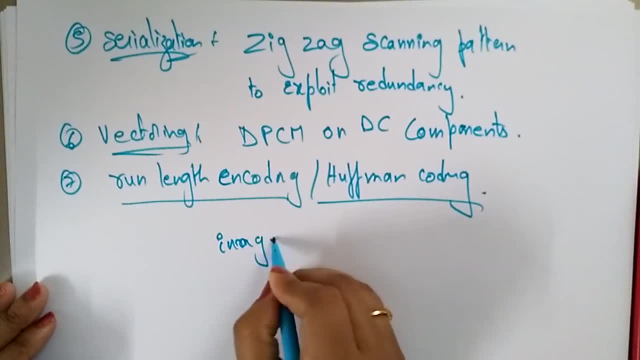 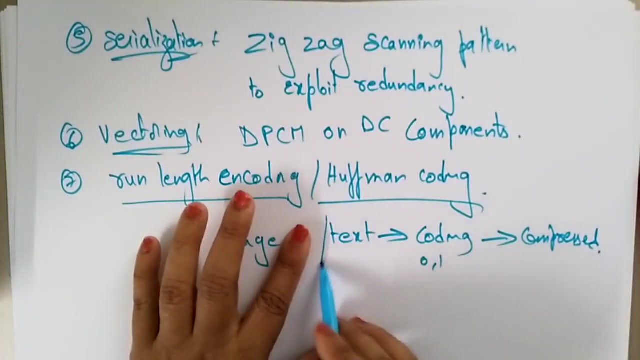 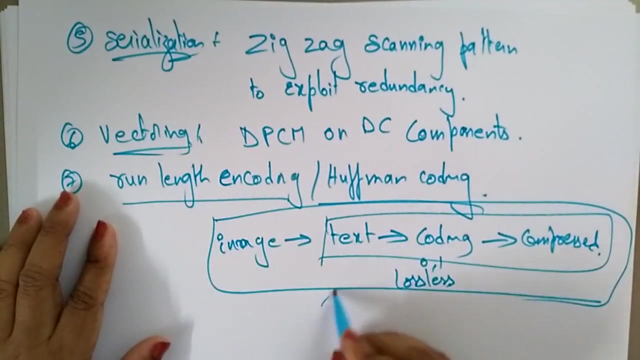 so first thing is, whatever the image that is there that you need to be converted into text. after that, apply the uh coding means convert into zeros and ones and then compressed. so this is so so far. we have seen this technique in the lockless, so here, lossy, this is lossy. 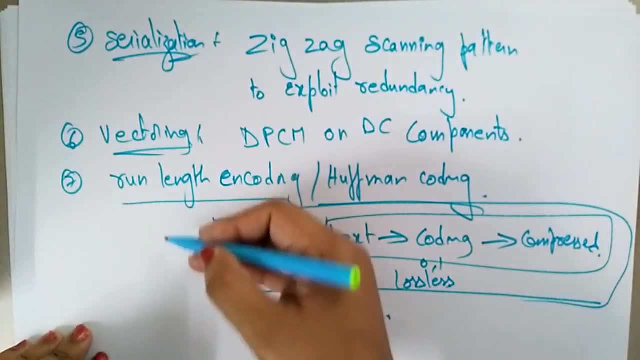 so here the image has to be changed, so you have to follow all six steps to convert the image into text. okay, so this is about this, uh, jpg schematic. so in the next video i will explain with an example so that you clearly understand what exactly the jpg- anything exactly. coding boss, thank you.